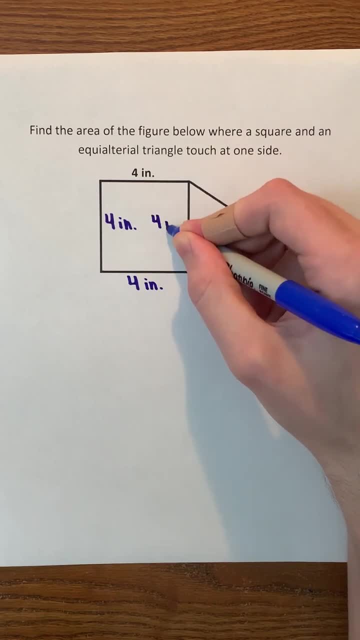 Therefore, all of these sides must also be 4 inches. Also, in an equilateral triangle, all of the sides also have the same length. Thus, because this side is 4 inches, all of these other sides must also be 4 inches. 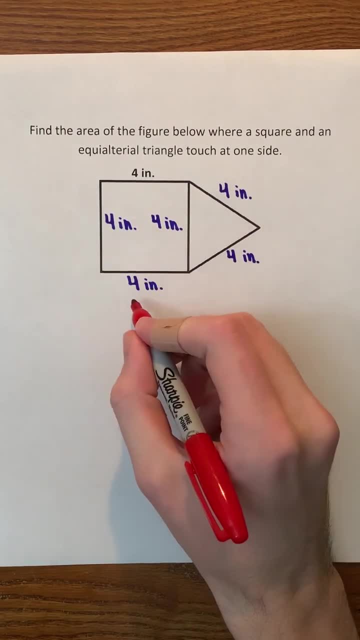 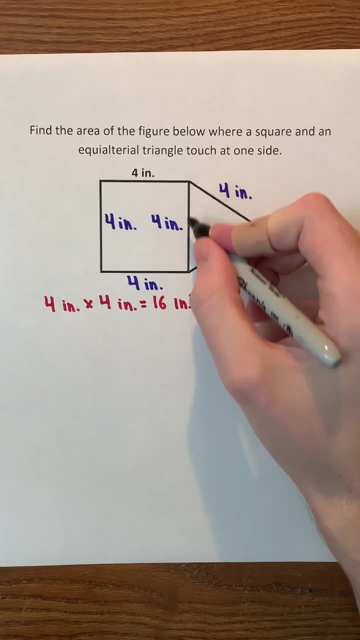 Now we can find the area of the square. by multiplying 4 inches by 4 inches to get 16 square inches. Next we're gonna find the area of the triangle where we need the length of the base, which is 4 inches in this case. 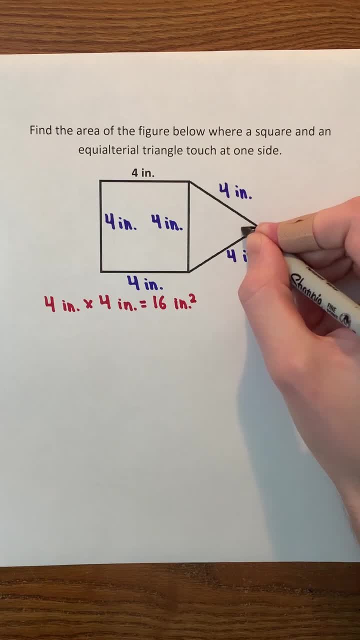 and we need the length of the height. but we don't have that right now, So we're gonna find it by first drawing this line right here which bisites the triangle into two congruent right triangles. Thus this angle right here must be 90 degrees. 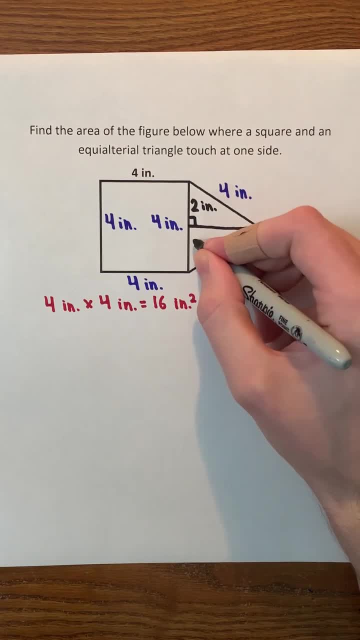 and this side length must be 2 inches. In addition, this side length must be 90 degrees, must also be 2 inches. 2 plus 2 is 4.. Now we're gonna use the Pythagorean theorem to find the height. So we're gonna have 2 squared where 2 is the length of this side. Then 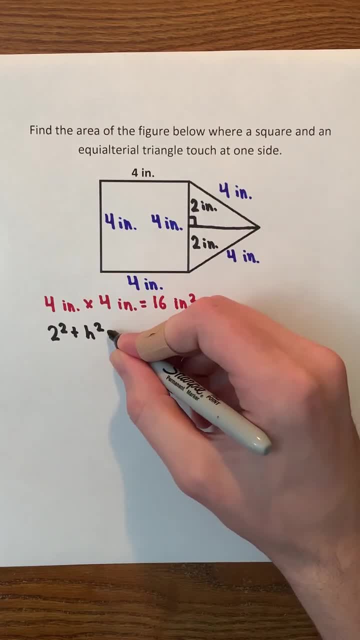 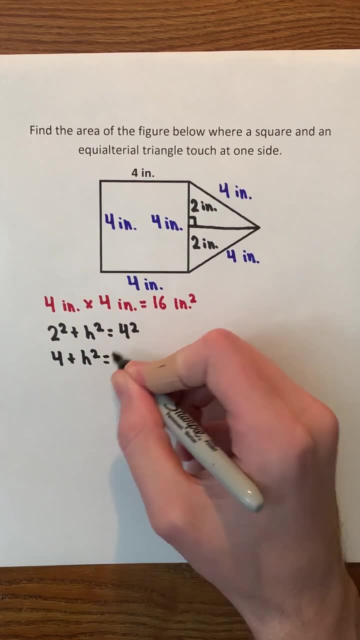 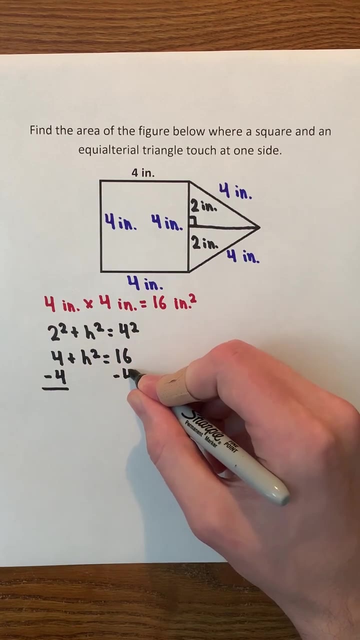 we're gonna add h squared where h is the height. Lastly, we're gonna set this expression equal to 4 squared where 4 is the length of the hypotenuse. 2 squared is 4, and 4 squared is 16.. Now we're gonna solve for h by first subtracting 4 on both sides of the equation. 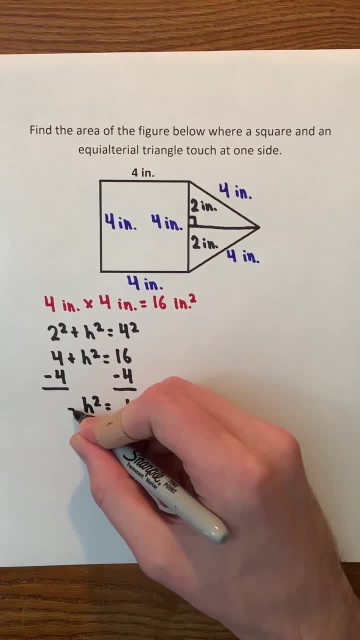 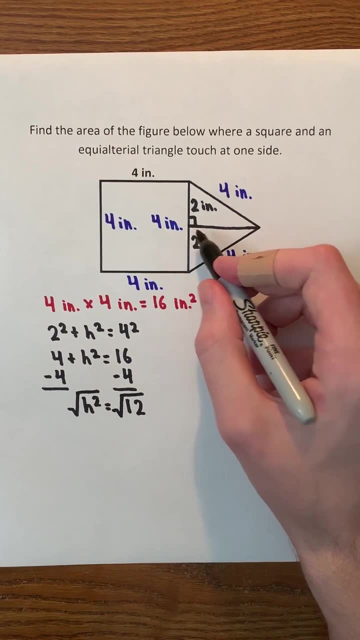 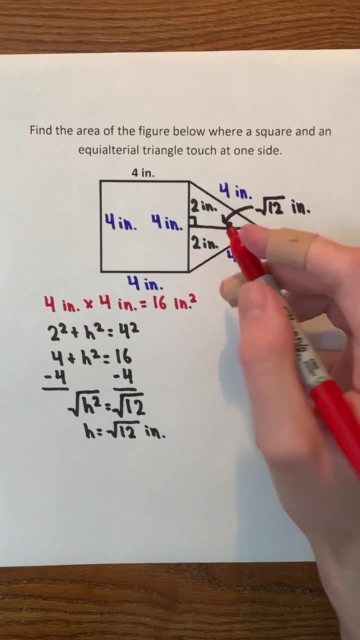 And we get h squared equals 12.. Then we're gonna take the square root of both sides. We don't need the plus minus next to the square root of 12, since the height is positive. Therefore, the height has a length of the square root of 12 inches. Finally, we can find the area. 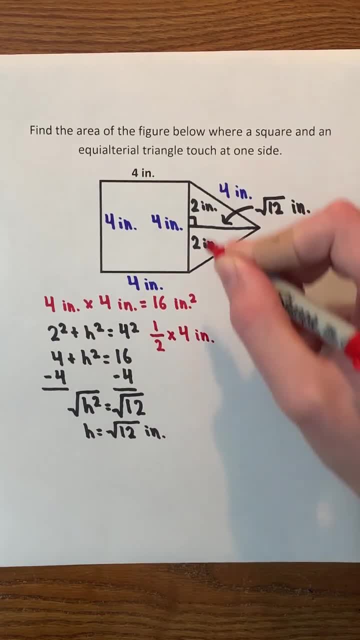 of the triangle by multiplying 1 half by 4 inches, where 4 inches is the length of the base, And then we're gonna multiply by the square root of 12 inches, where the square root of 12 inches is the height. 1 half times 4 is just 2.. So the area of the triangle must 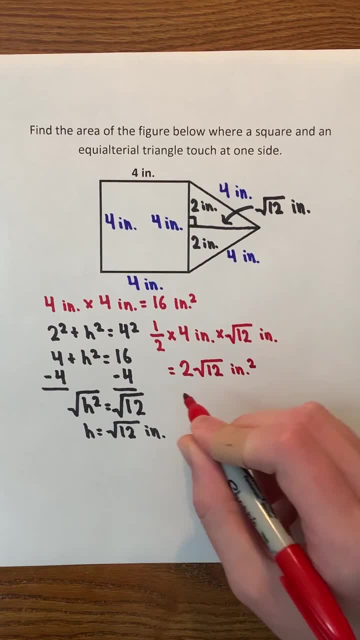 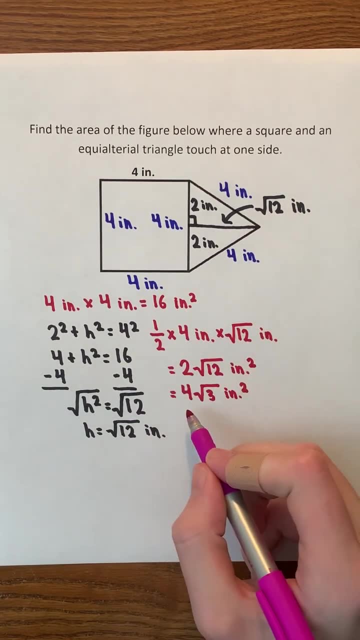 be 2 times the square root of 12 square inches. We can simplify this to 4 times the square root of 3 square inches And the final step is to just add the area of the square and the area of the triangle. So we're gonna have 16 square inches plus 4 times the square.